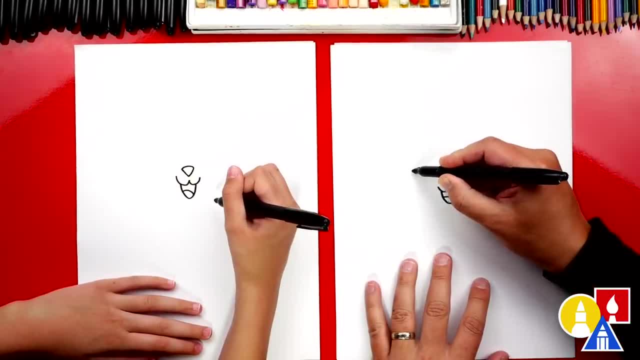 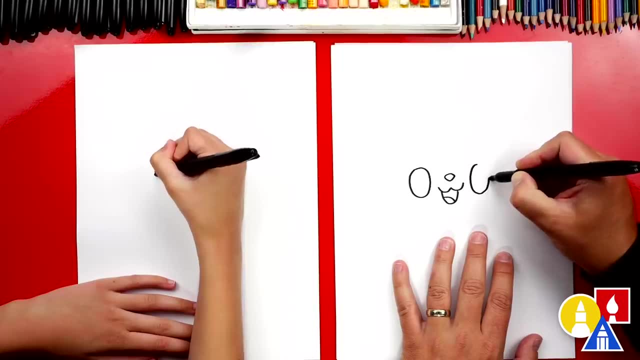 Now let's draw the eyes And instead of drawing a circle, let's draw big ovals. We're going to draw about that size- Whoa, really big. And then another one the same size over here for the right side- Ooh, really big. 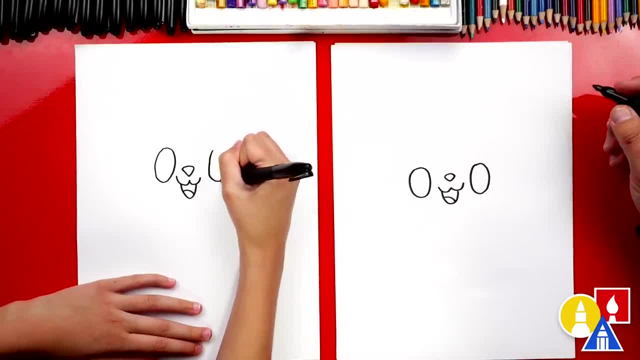 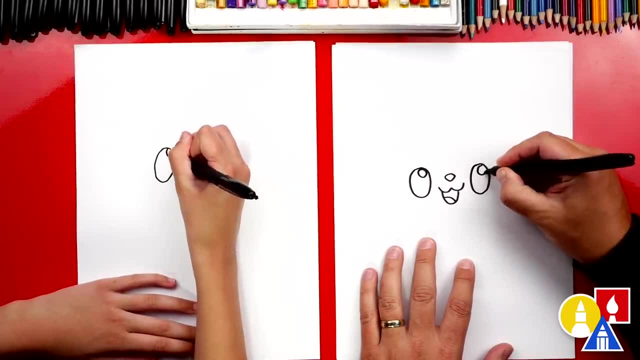 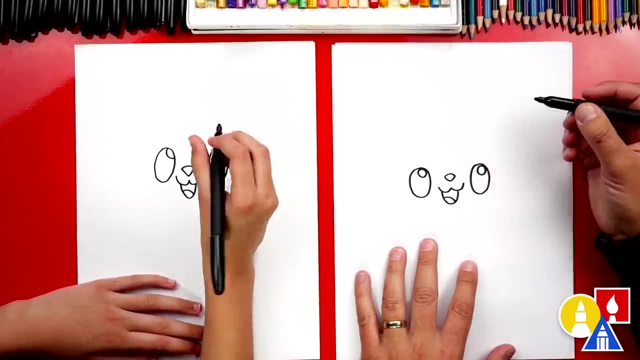 Really big. Those are super big. Okay, now let's draw a circle in the top right for the highlight in each eye, And then this part. we're going to fast forward, but we're going to color in the big oval but leave the little circle white. 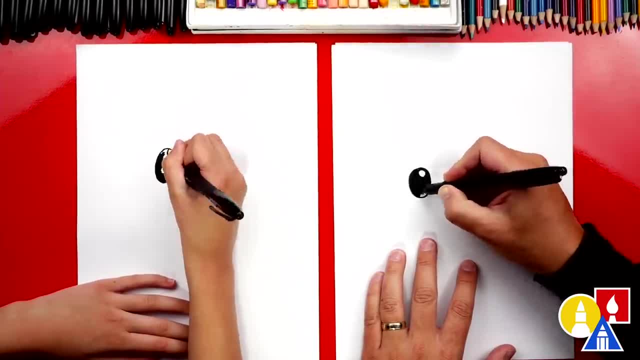 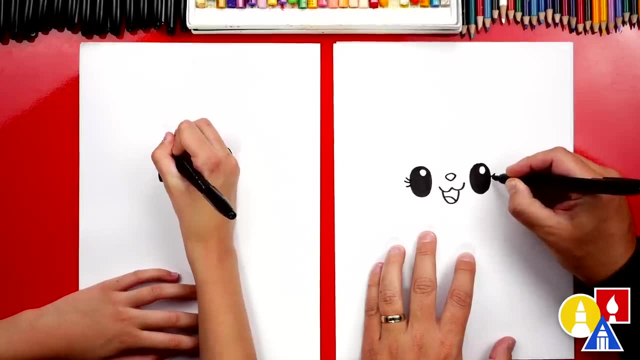 Now, if you need more time, remember, you can always pause the video. What should we add next? Eyelashes. Yes, we can add three little eyelashes: Eyelashes on each eye, or you could add more if you want. 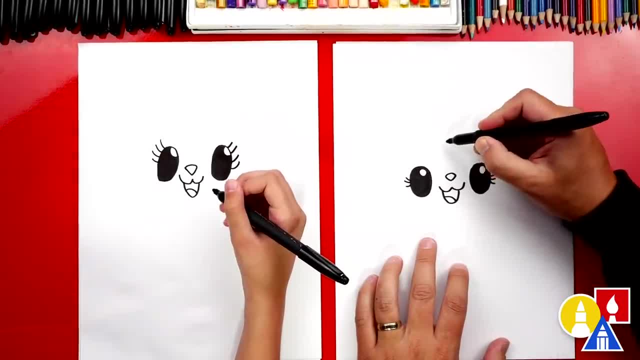 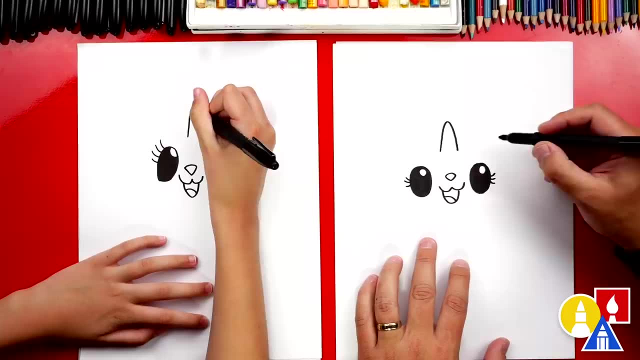 Now, what should we draw? The horn, The unicorn horn. Okay, we'll draw an upside down v right above the nose And then down at the bottom. let's draw a little curve to connect. Kind of looks like an upside down carrot. 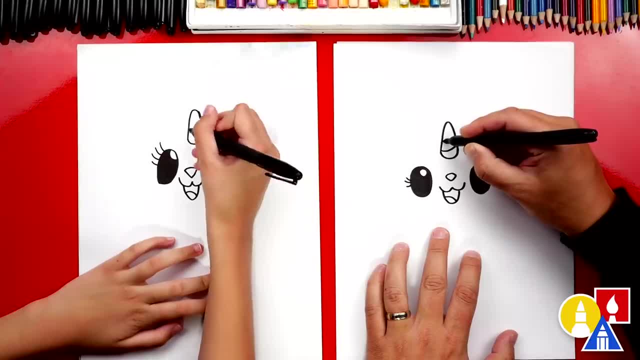 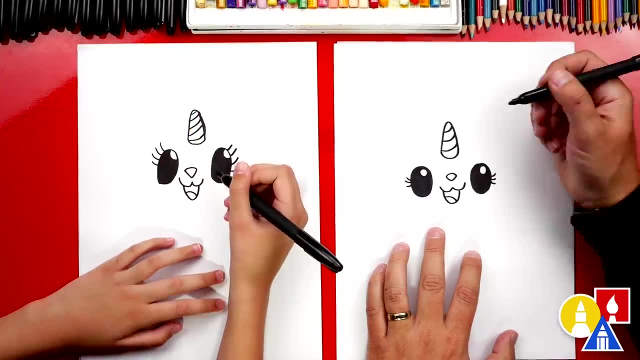 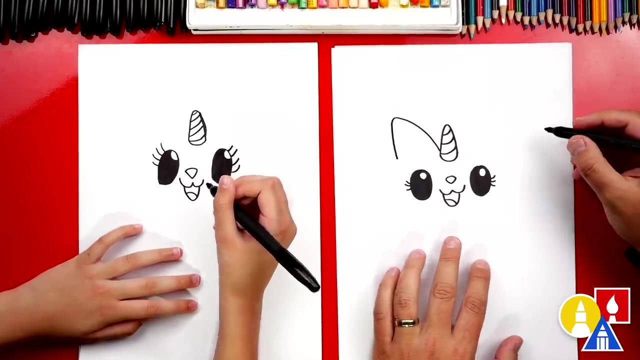 Okay, we can also draw the texture on the horn. I'm going to draw little curves going across the top. Now let's draw the ears. We could draw an upside down v coming up and then back down. Those are big ears. And then we're going to do the same thing on the other side. 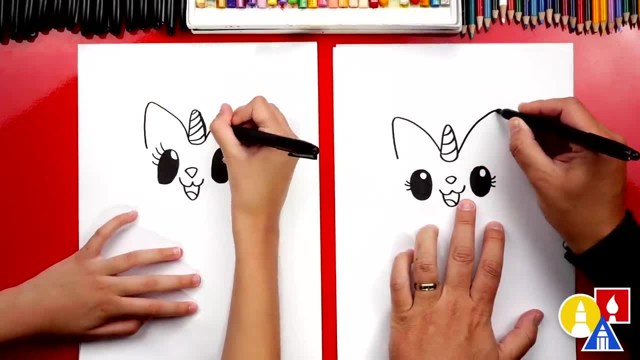 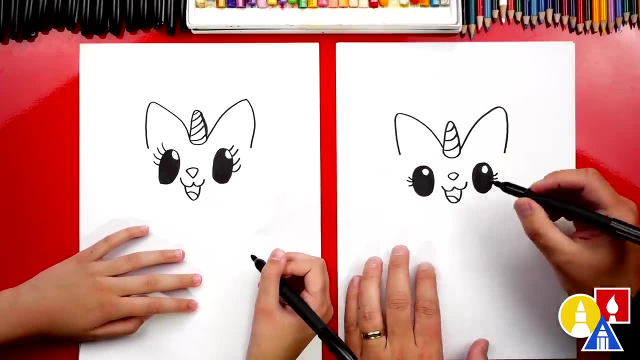 We want them to look the same on both sides, So try to match the same height and we'll come down to the same spot on each side. Now let's draw the shape of our cat's head. We can come down. we're going to draw the cheek, then we're going to come up and then we're going to draw the nose. 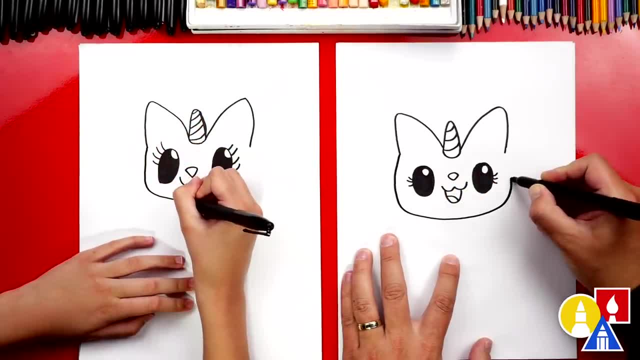 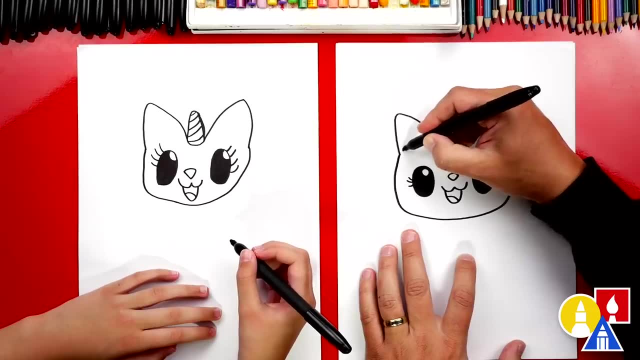 And then we're going to come under across and then connect up to the other ear. Next, let's draw the inside of our cat's ear. I'm going to draw the same shape that we first drew for the ear, but smaller, inside. 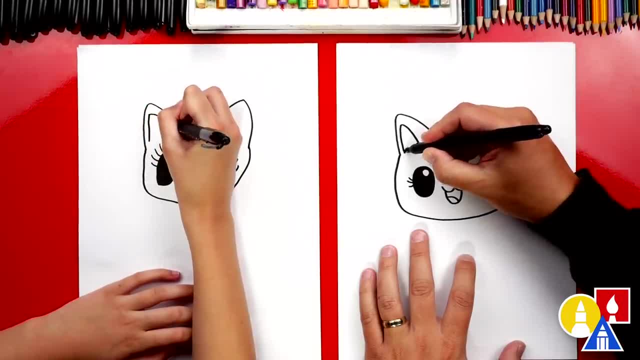 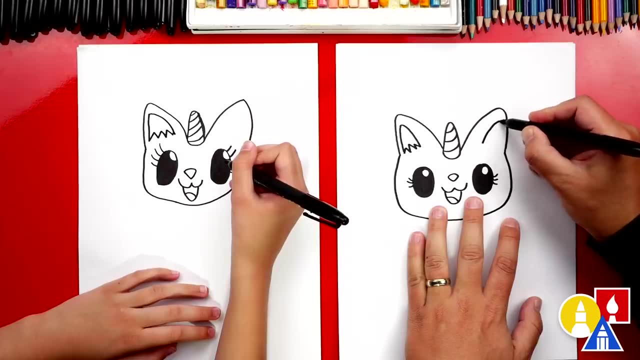 And then we can draw little zigzags to connect the bottom. Now let's do the same thing over here for the right ear. We'll come up, back down and then zigzag At the bottom. Oh, I just connected it. 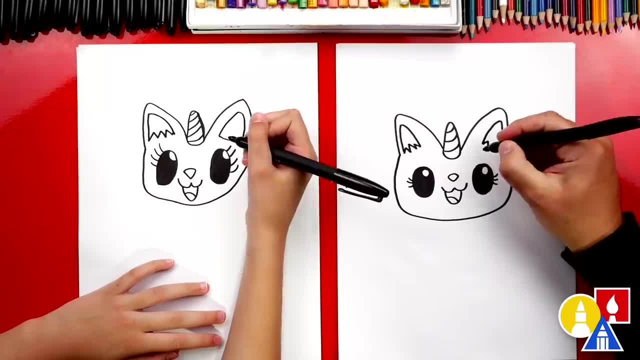 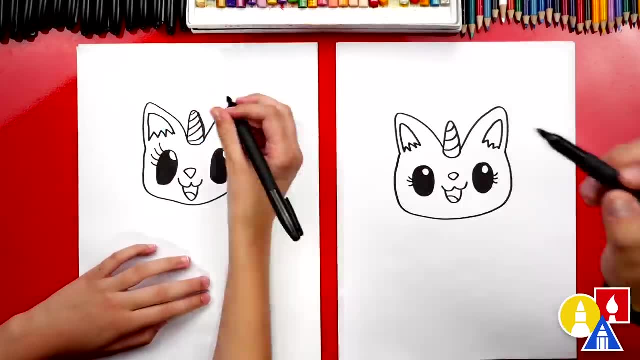 Oh, I like it. That's okay, right, There's no mistakes. You could even add zigzags on top of that if you wanted. Yeah, just like that. That looks cool. You could also add a line on this side so that they match. 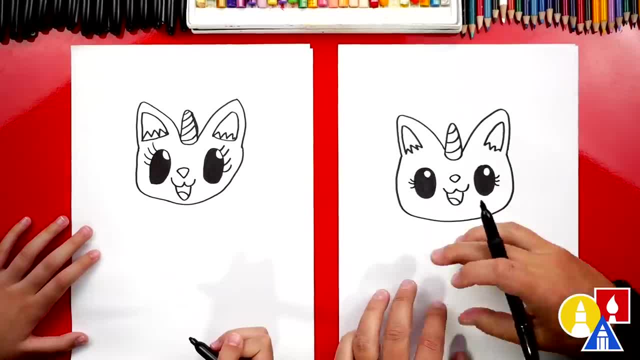 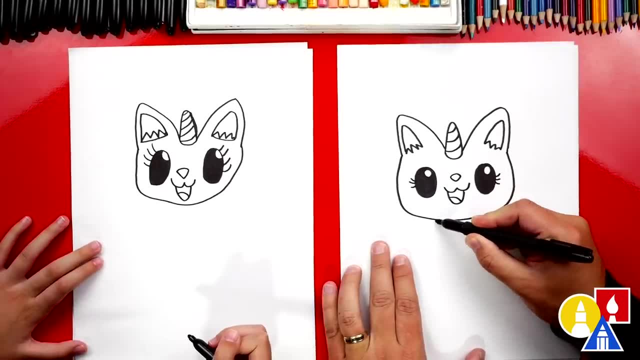 Yeah, I like that. Oh, that's cute. Okay, now let's draw the body. and we're going to draw our unicorn jumping through the air, Or a cat unicorn, Okay. so let's draw the body first. We're going to draw. we'll start here, on the chin, and we're going to draw a curve that comes down. 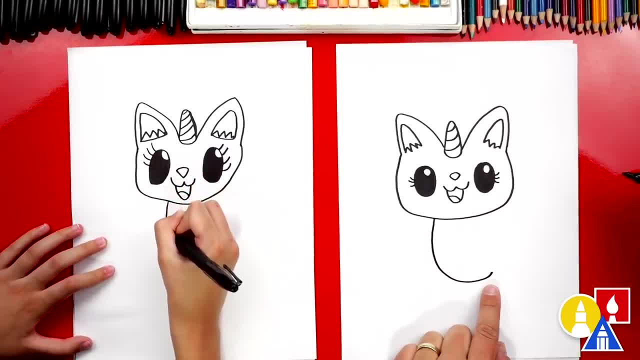 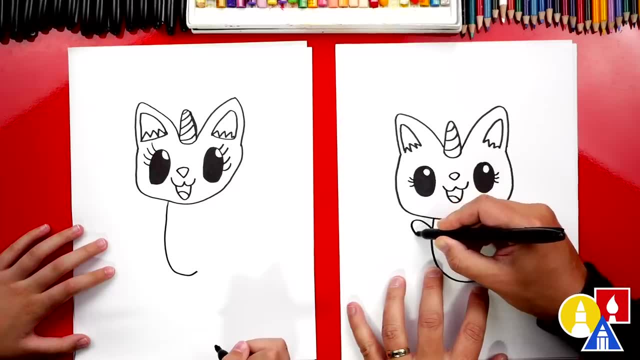 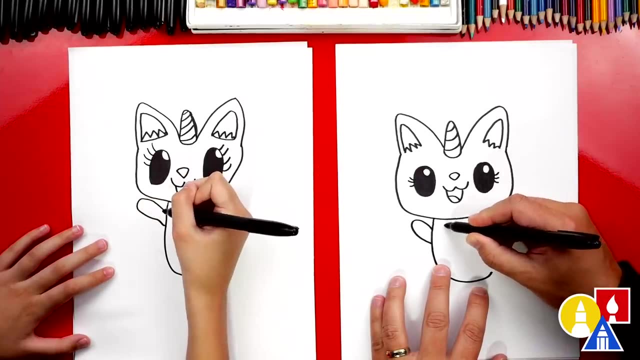 and then starts curving back up Right. at the end. Let's draw the arms, the front legs. We'll draw an upside down? U coming up to the left and then let's draw another upside down U inside of the body, like right here. that matches. 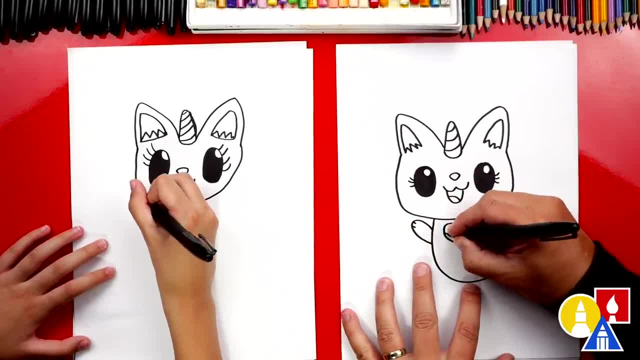 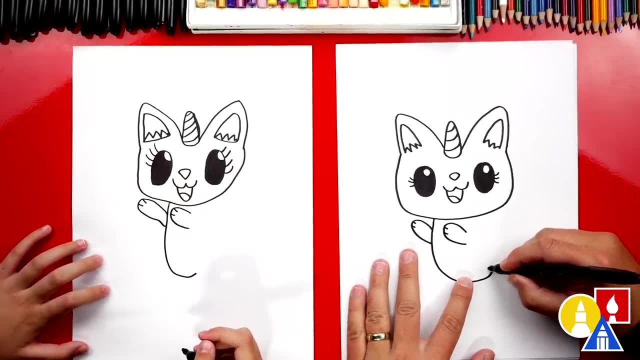 Then we can. let's add two little lines for the fingers or the paws. Now let's draw the back leg. We're going to start here inside the body. We're going to curve down and then back up. We're trying to make the back legs look kind of like the front legs too. 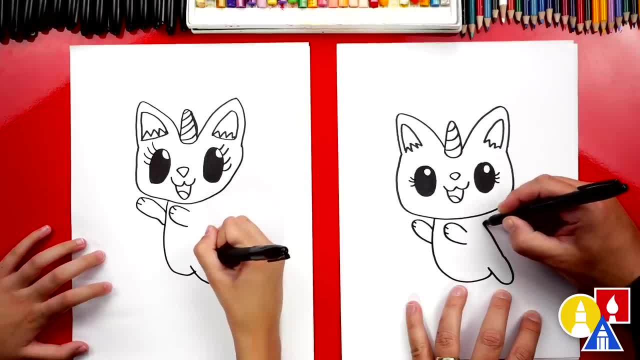 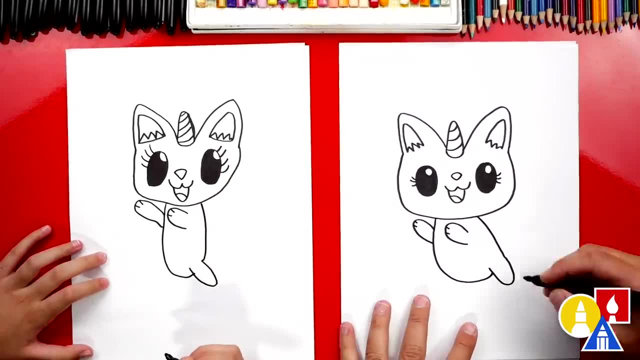 And then right here at the end, we can curve up and connect into the body. Yeah, just like that, That's a skinny body, I like it. And then we can also add two little toe lines for that foot. And then let's add another leg right here. 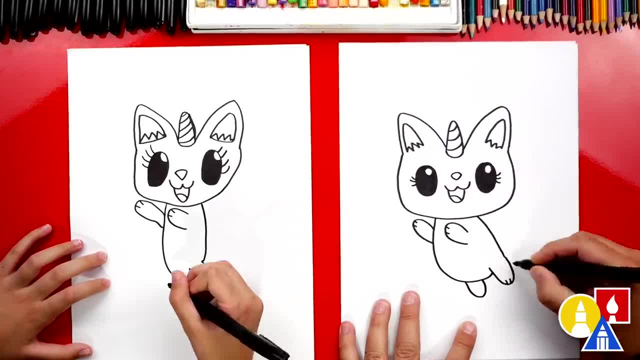 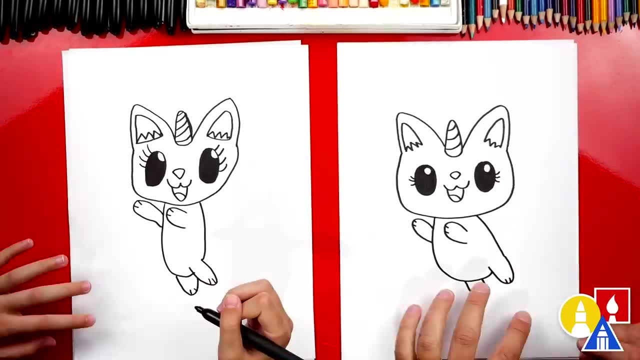 That matches So the same size U shape. And then let's draw two little toe lines. Now let's draw the really cool tail. Let's start here. We're going to draw it really big. We're going to draw an S curve. 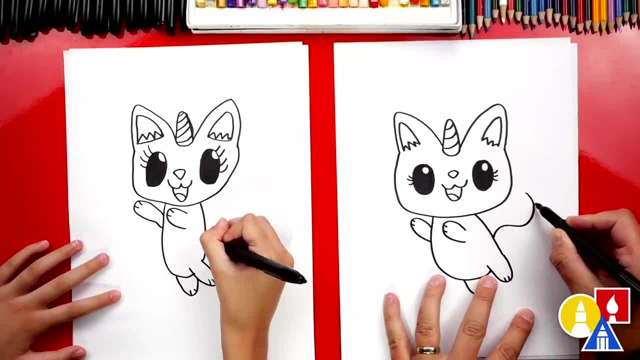 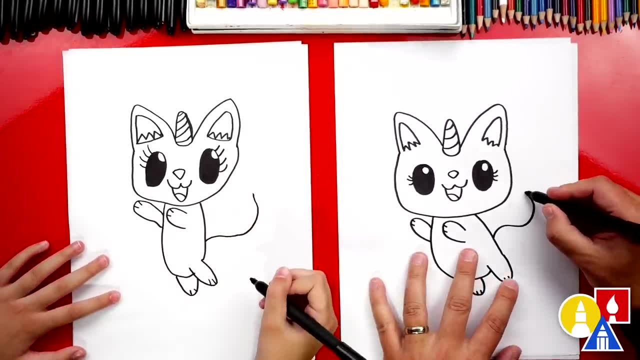 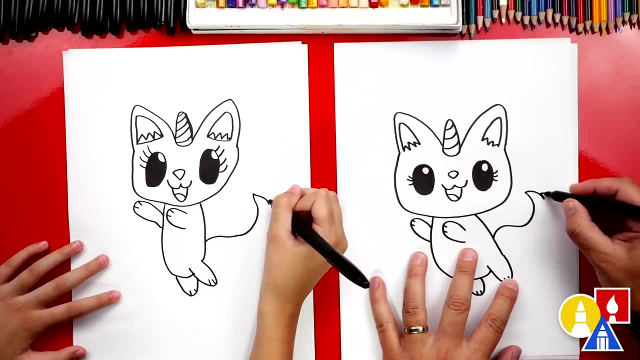 So you can draw curving up, then curving back down and curving back up. Yes, Then we can add the other side of the tail. We'll curve This way. Then let's add a little zigzag line back up and we'll curve down further. 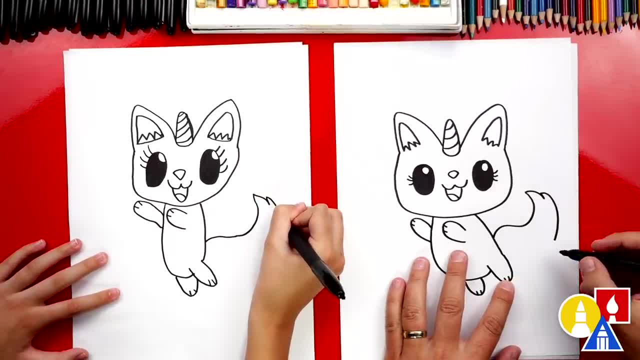 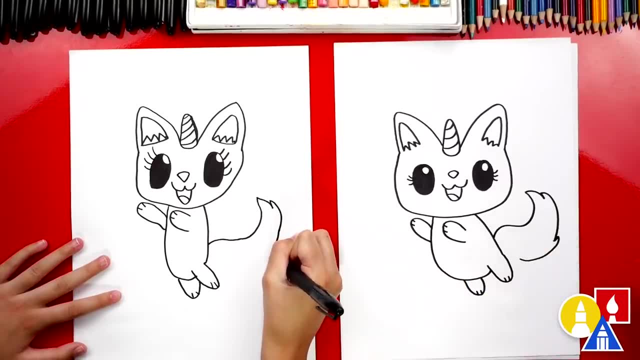 And I'm going to get further away- Look how thick my tail is getting. Then we can add another little zigzag line and curve down further. And let's add one more little zigzag and then connect it into the body. We have one more thing to add, and that's the whiskers. 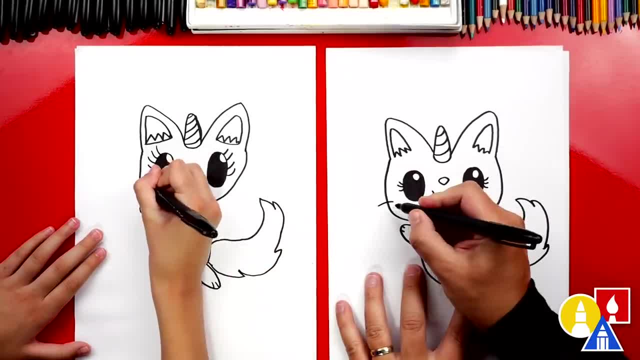 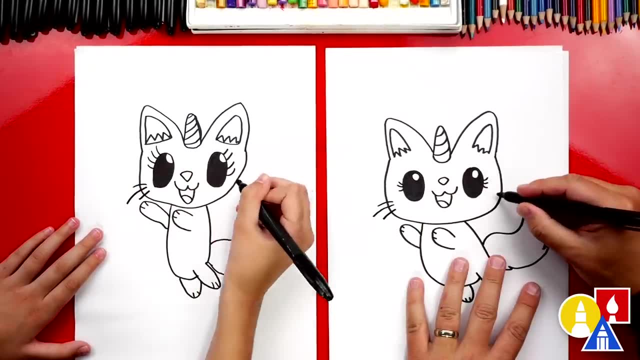 I'm going to draw one curve coming out of the cheek, Then I'm going to draw a longer curve coming out further and then a shorter one below that. Let's do that same thing on the right side: Short: one long whisker and a short whisker. 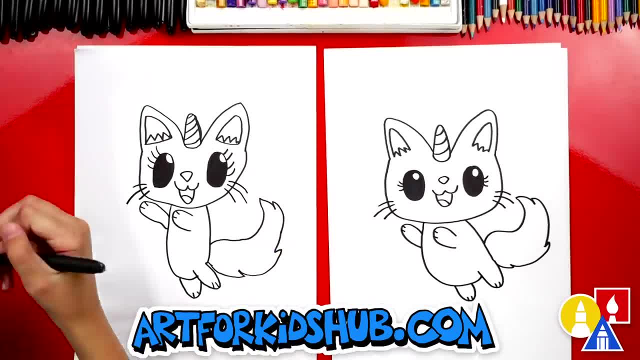 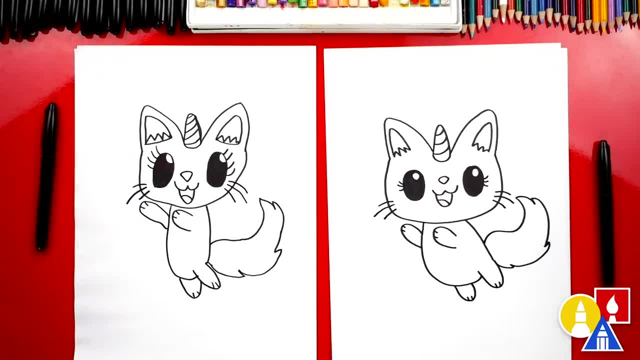 Hadley, we did it. We finished drawing our unicorn kitty, or our cat unicorn, Yeah, Except we still need to Color it. This part we're going to fast forward, But at the end you can pause the video if you want to match our same coloring, or you can color your cat. 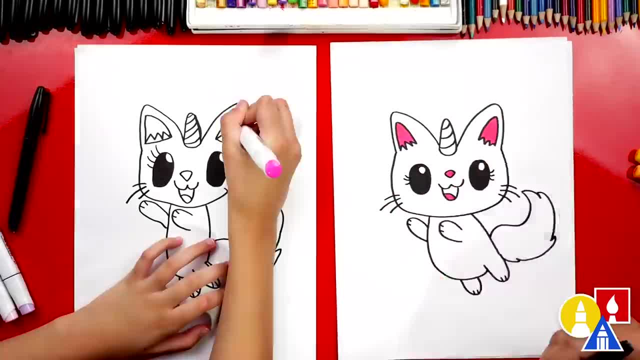 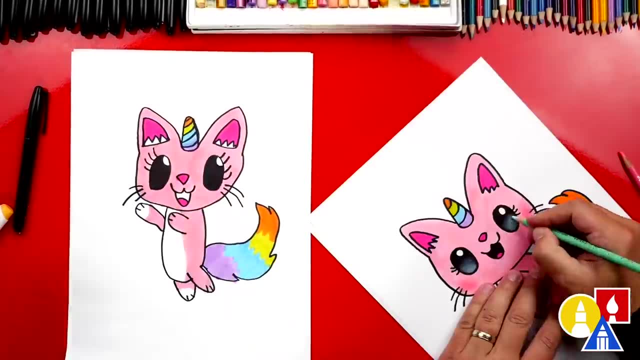 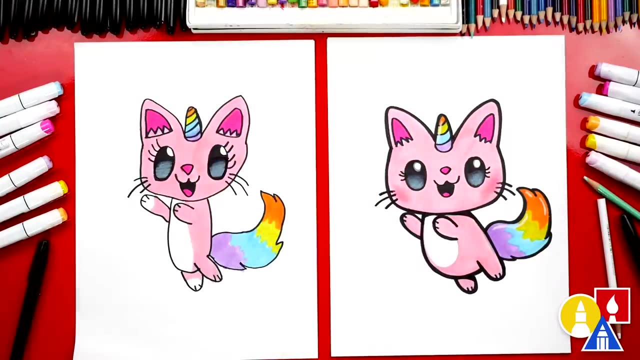 Cat unicorn. Any way, you want You ready to fast forward? Yeah, Hadley, give me five. We did it. We finished coloring and drawing our cat unicorn. I love how it turned out. Did you have fun? Yes, You promised. 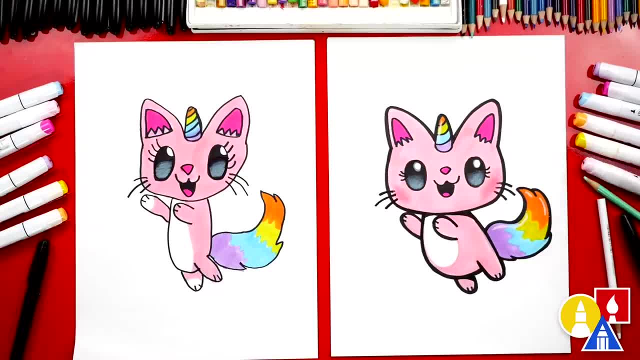 What do we use to color our drawings with Markers? Yeah, we use our biannual markers. If you have the same set, we use R502.. R502.. R502. R502. R502. R502. R502.. 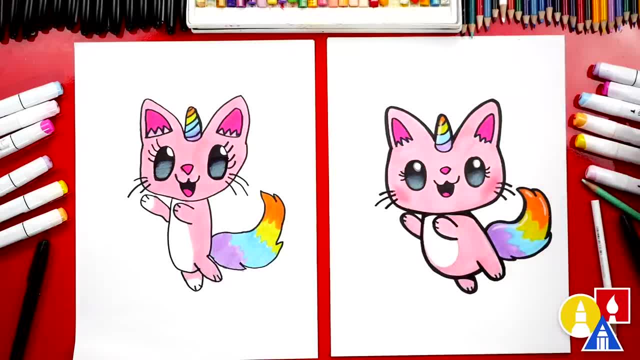 We used the same color of our cat and then we used our yellow, orange, blue and a bright pink- Also a purple, to color the rest of it. But you don't have to color it the same way that we did. You could color it your own way. 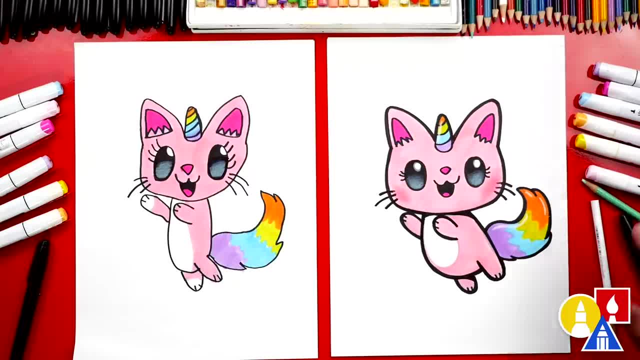 Yeah, You could also use Cranza Oil pastels. Yeah, You don't have to use our markers. Yeah, One of my other favorite things that we did was we added another reflection on the bottom of the eye to make it look even shinier. 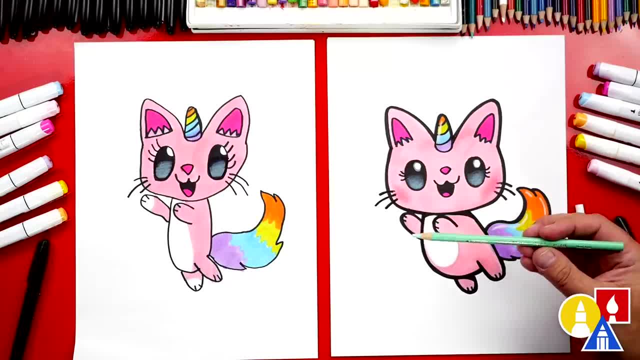 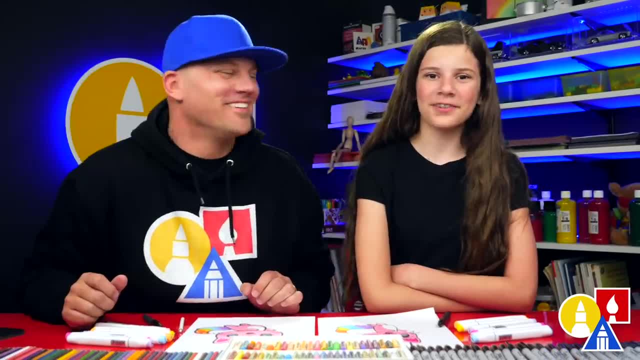 And cuter And cuter. Of course, yeah, We used our Prismacolor colored pencils. The color is Deco Aqua, But you can use whatever you want. You could use any color, a light color, for that reflection. We hope you had a little fun drawing your cat unicorn. 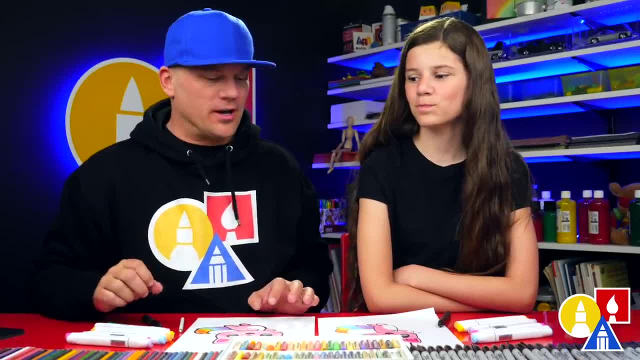 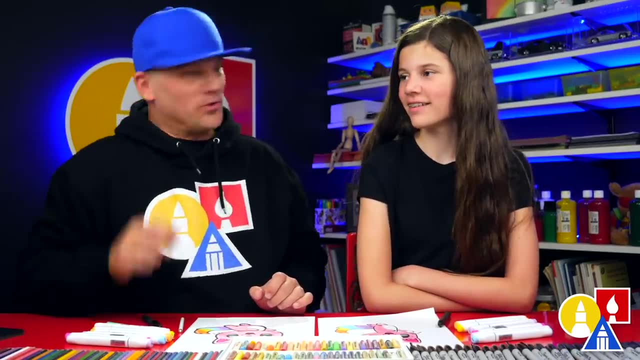 We do and we hope you take extra time to add even more things to your drawing in the background. Maybe you could add clouds Or a rainbow- Oh, a rainbow would be really cool- or even more cats with horns Jumping out of a rainbow. Yeah, And we'll see you later. art friends, Goodbye, Goodbye.